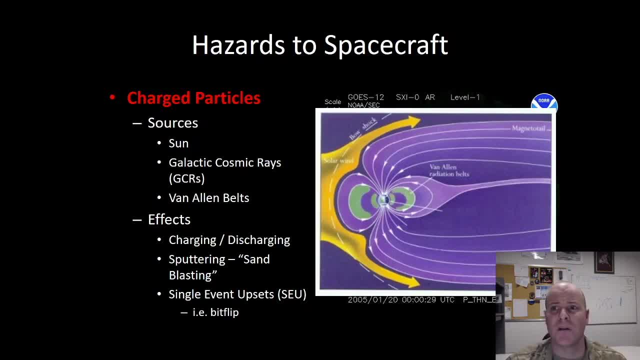 Charged particle effects may be in the form of rapid charging or discharging of our spacecraft, sputtering or sandblasting from high-speed particle impacts, or bit flips, or also known as single event upsets, which may harm satellite electronics. 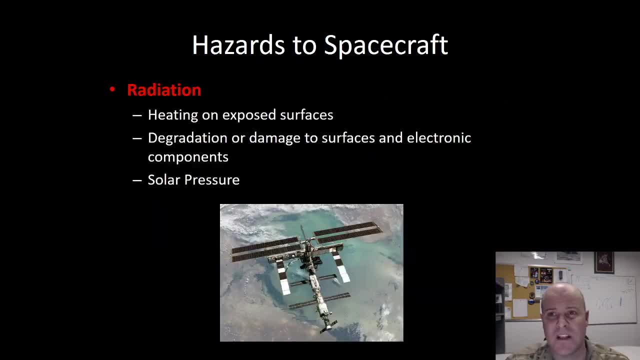 Our next hazard is that of the radiation environment. The radiation environment from the sun can heat expose surfaces, which is generally pretty good for solar cells when it comes to power, but it can be bad for electronic components and the cells themselves if the heat is too much. 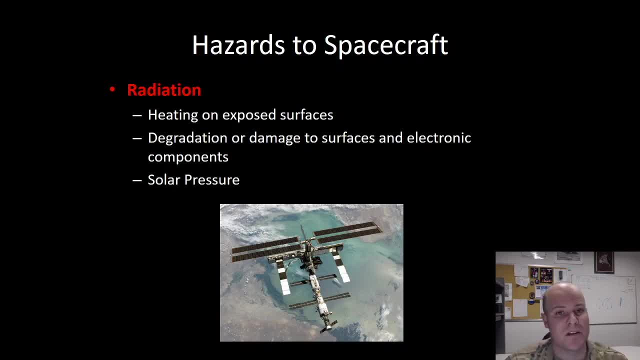 It can also degrade spacecraft coatings, particularly on solar cells, over time. Solar pressure is caused by photons and is very small when compared to drag. However, over time, it can upset a spacecraft's orientation, causing it to point in the wrong direction, which is definitely a hazard. 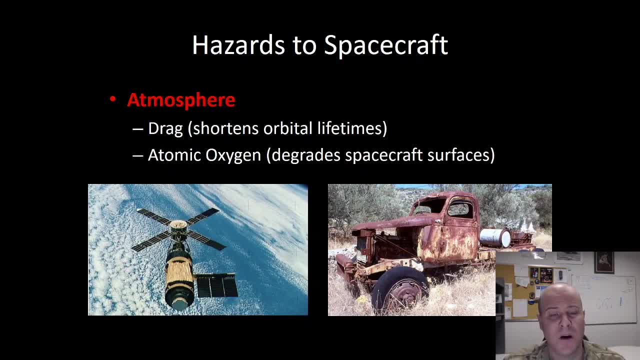 Our next hazard is that of atmosphere. The particles in the atmosphere can cause drag. The effect of drag on our satellite is variable depending on the orbital altitude and spacecraft size. Between 130 and 600 kilometers it varies considerably, while above 600 kilometers the effects of drag were pretty minimal because the atmosphere is so thin. 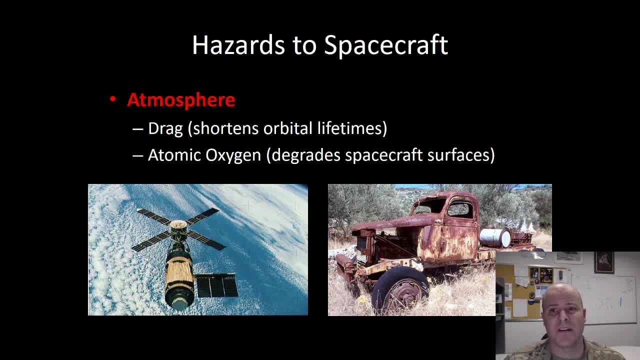 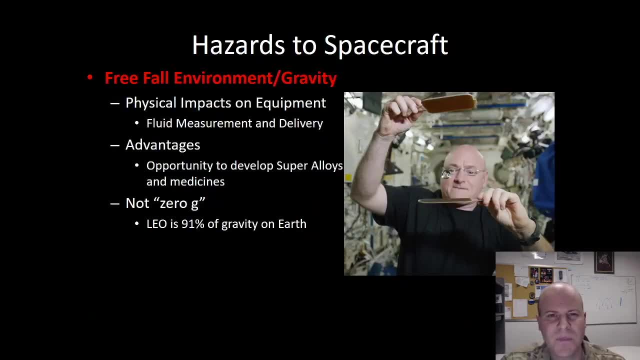 Atomic oxygen from the atmosphere can also degrade the spacecraft's surfaces as it oxidizes, much like it does on Earth. Our next hazard is that of freefall. The freefall environment for our spacecraft means there are no contact forces, which is good for our experimentation and mixing of materials. 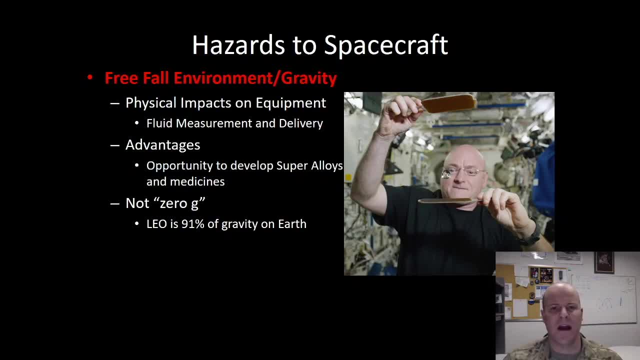 However, it can be frustrating for engineers, as it's hard to know how to handle liquids exactly in that environment. Notably, the spacecraft is in freefall around the Earth in its orbit, not in zero-g, as often incorrectly stated. Our next hazard is that of vacuum. 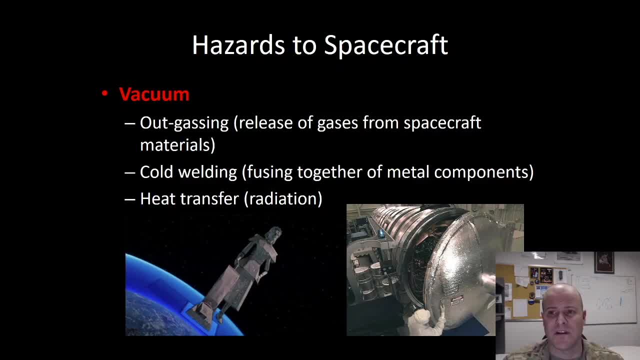 The vacuum of space will cause outgassing for our satellite. The ambient pressure in space is nearly a perfect vacuum. This greatly reduced atmospheric pressure causes some materials to release trapped gasses. For this reason we often bake our satellites in thermal vacuum chambers prior to flight. 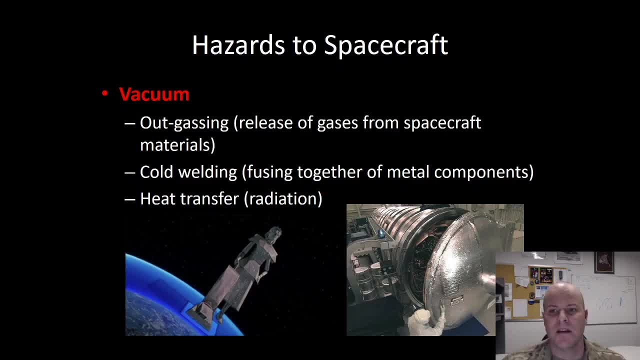 to mitigate the inevitable outgassing in space. Cold welding is another really interesting phenomenology that only occurs in space. Cold welding occurs when mechanics or mechanical parts that have very little separation between them get up into space. This pocket of air disappears due to the vacuum of space. 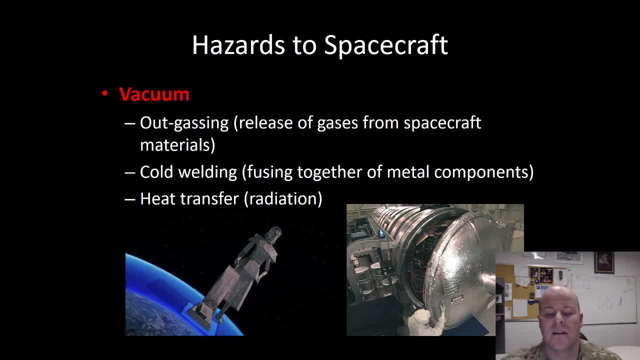 and essentially causes the parts to fuse or weld together. For this reason, satellite designers try to avoid using moving parts where they can. Another interesting effect of the vacuum of space is that of having only radiation as a heat transfer mechanism. Convection and conduction occur through a medium. 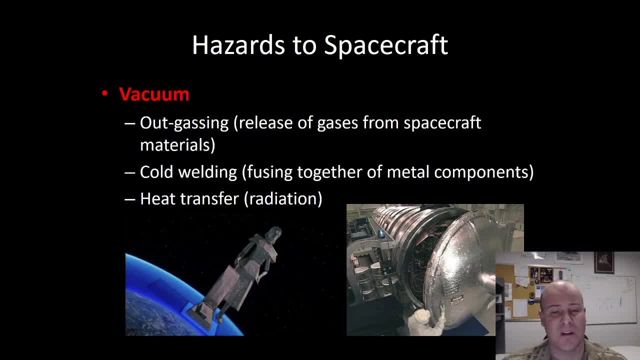 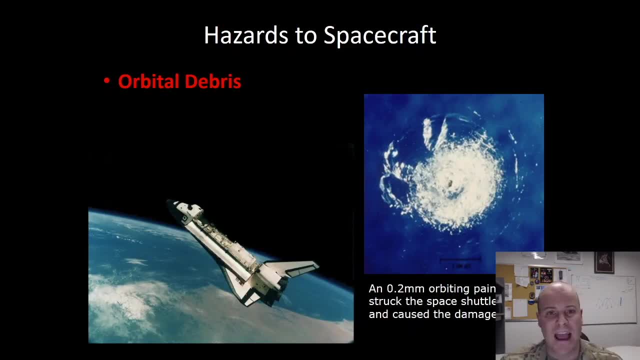 such as air or water. Since space is in a vacuum, radiation is the only method of heat transfer, which limits the effectiveness of the satellite to get rid of excess heat. Our last hazard that we'll talk about in space to our spacecraft is that of orbital debris or space junk. 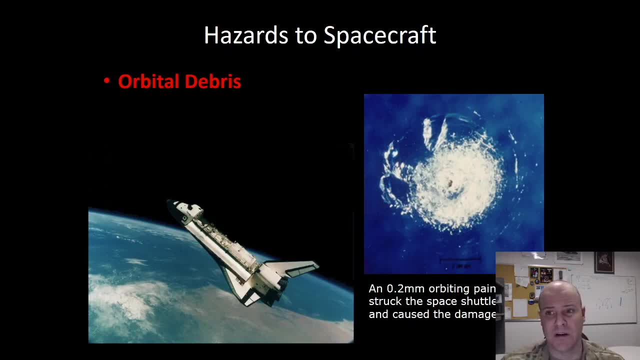 Micrometeoroids or space junk or orbital debris- all the same thing can damage a spacecraft during a high-speed impact, Even things very small, such as an orbiting paint chip, which, as you can see here, is a depiction of in this picture. 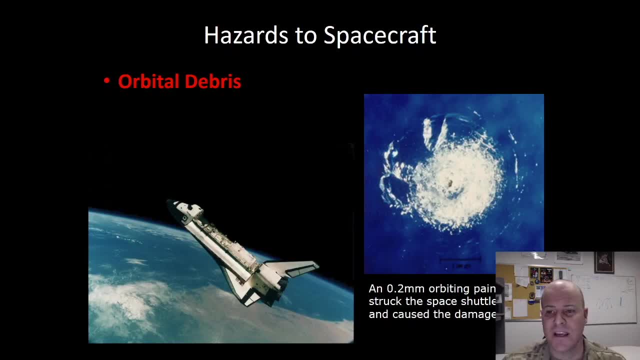 In this case, an orbiting paint chip struck the space shuttle in 1983, causing this kind of damage that you see. The paint chip was only 0.2 millimeters in diameter, but was traveling around 30,000 miles per hour when it hit. 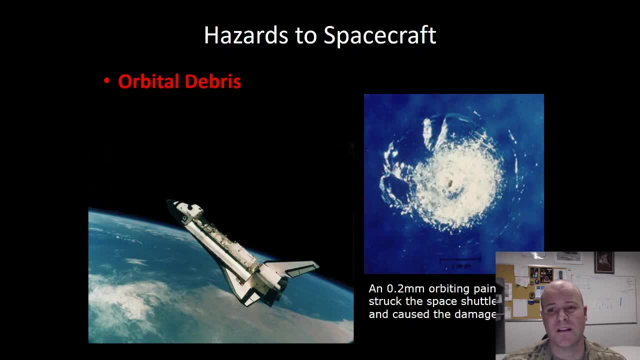 causing a 4-millimeter wide crater. that's about 20 times its original size. You can imagine the kind of damage that you could expect from something even larger, such as like a baseball or even a softball, or even larger. It could absolutely devastate your spacecraft. 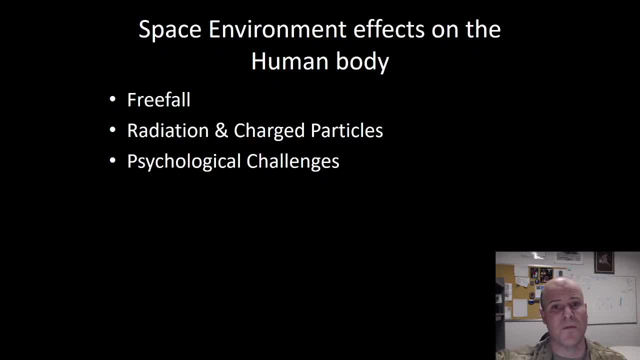 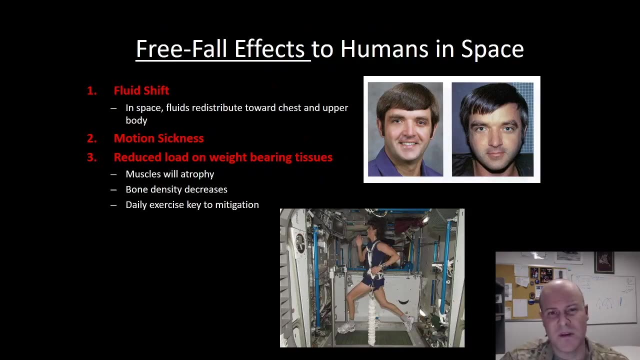 The space environment also has effects on the human body, not just our spacecraft. We're going to talk about those here now, Essentially freefall effects, radiation-charged particle effects and also the psychological challenges. First, freefall: Some effects on the human body due to freefall. 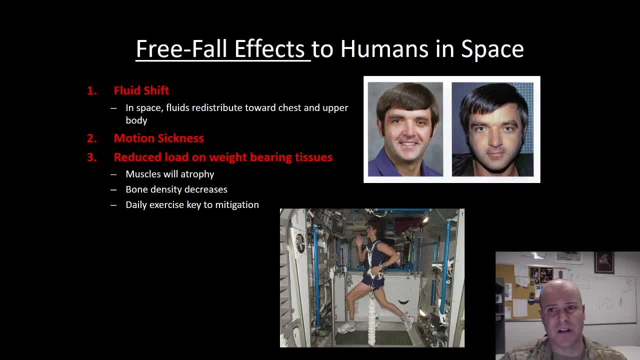 are that of fluid shift In space. your fluids are going to redistribute all around, primarily toward your chest and upper body. It can cause even noticeable changes in people's appearance, such as what you might see here in this picture over here to the right.